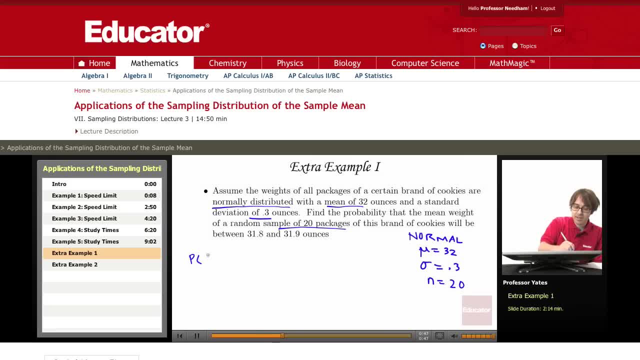 is 20.. So we're trying to find the probability that the sample mean is going to be between 31.8 and 31.9.. Because it's a normal distribution I could standardize. I could standardize these and use z scores to find the probabilities. So I'm taking 31.8. 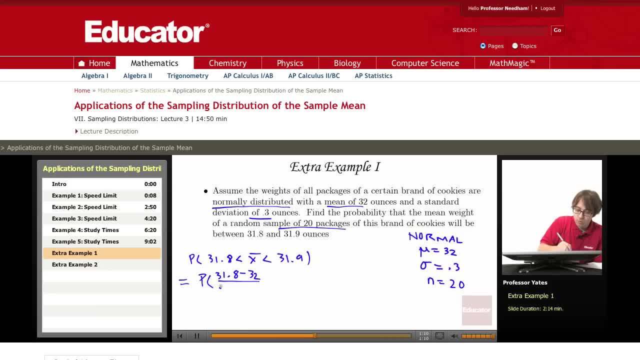 minus 32, divided by 0.3 over the square root of 20.. Z, and then we have 31.9 minus 32 over 0.3 over the square root of 20.. Okay, this gives me: 2.98 is less than z, which is less than negative 1.49.. If we were to sketch this out here: 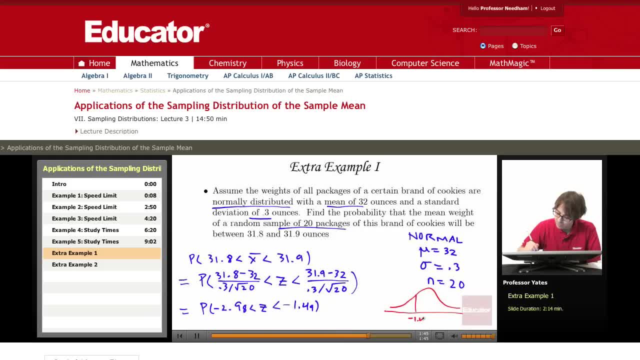 I have negative 1.49. And here I have negative 2.98. And I want the area in between those. So I look up negative 1.49 in the charts and that gives me 0.0681.. And then I look up negative 2.98 in the chart and that gives me 0.0014.. 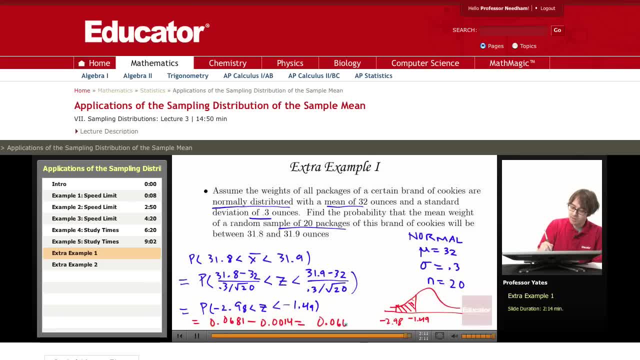 I subtract those two and I get for my answer 0.0667.. 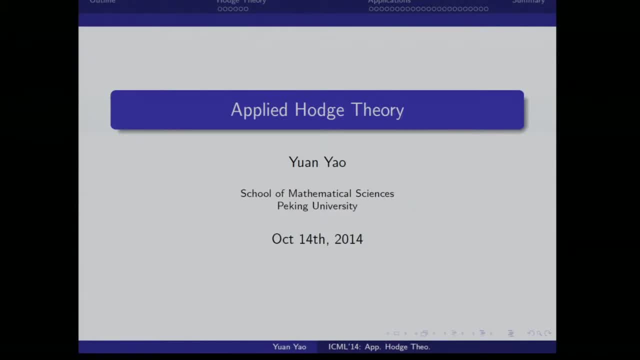 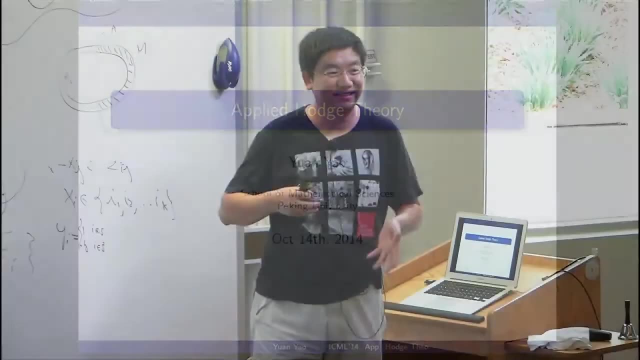 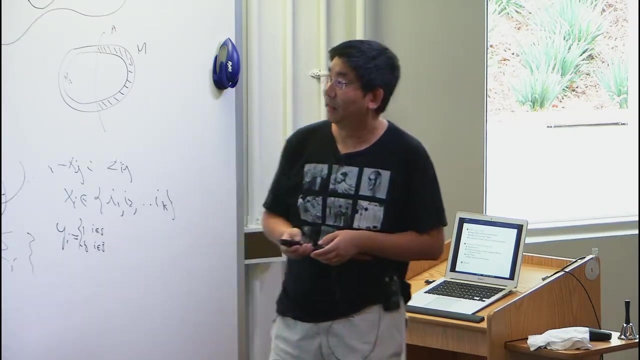 Thank you. Yeah, so sorry for the early starting. today I actually changed my slides because yesterday Lei-Heng pushed me to talk about hot theory and application, So somehow this is now the title appeared on the website, And what I'm going to show is this kind of. 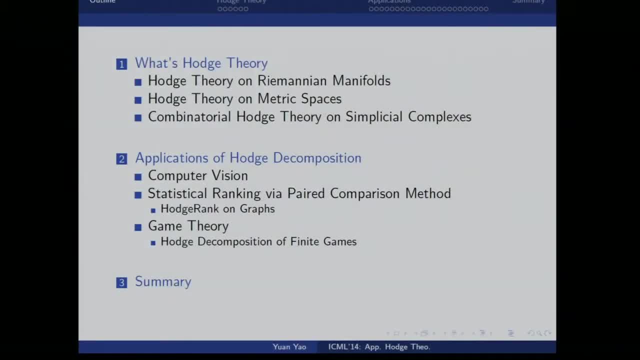 structure, Basically what's the hot theory? And actually Lei-Heng gave a very basic level, elementary introduction about that. So here I would like to point out the linear algebraic version of hot theory, together with various kind of pictures appeared in literature And